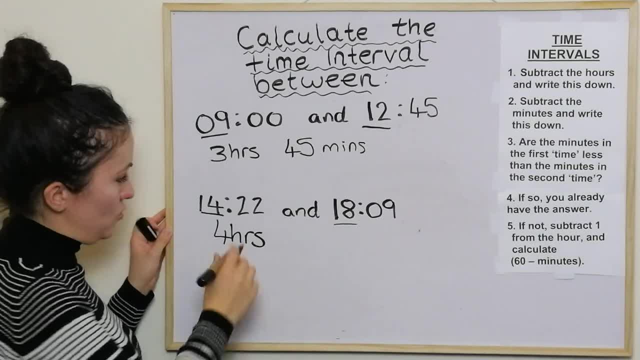 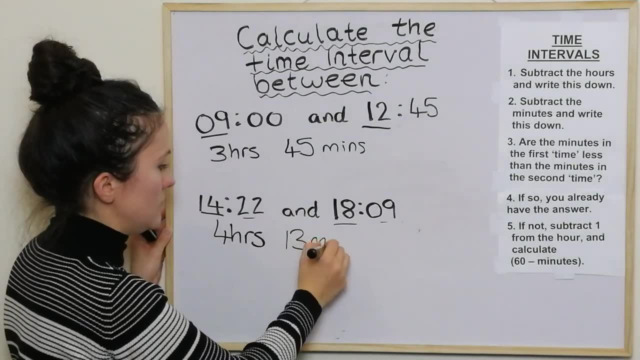 That's the hours, And then we subtract the minutes, So we've got 22 and we've got nine. So when we take those away from each other we get 13 minutes. So we've subtracted the hours, then we've subtracted the minutes. 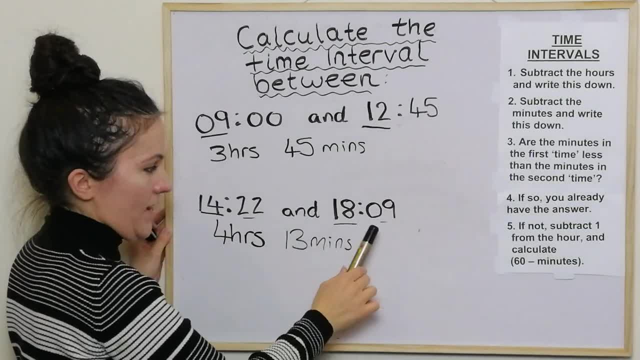 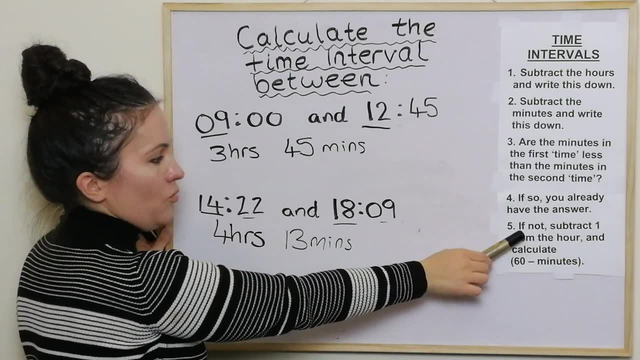 The next question asks: are the minutes in the first time less than the minutes in the second time? Well, the answer in that time is no, So we have to go in here. So what we do here is we subtract one from the hour. 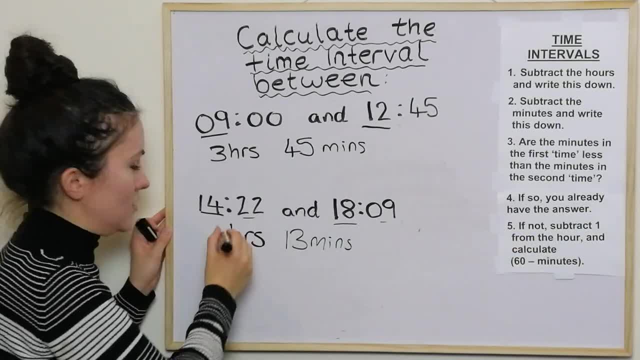 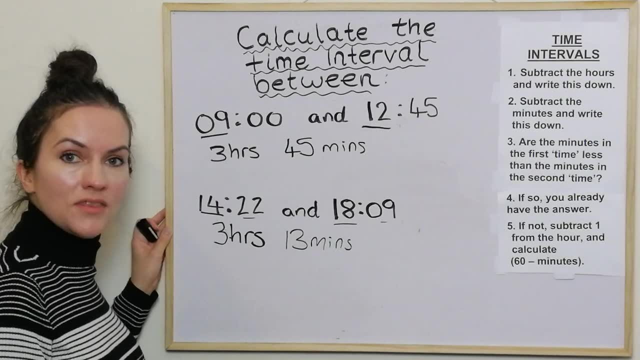 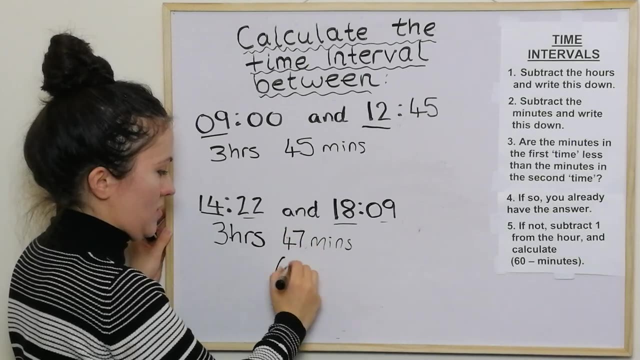 So instead of being four hours, it becomes three hours. And then we calculate 60, take away these minutes, So we do 60 take away 13,, which is 47. So 60 take away 13,, which is 47, and that's our answer. 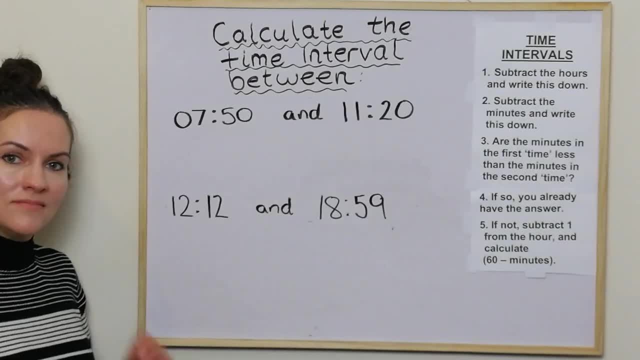 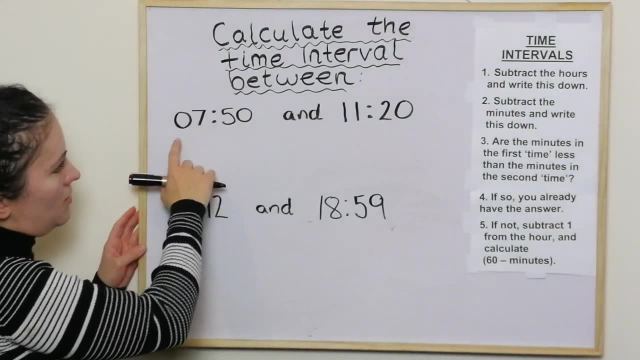 I'm going to do another few, Okay, this time, imagine this is fictitional. Imagine that we get on a bus from Glasgow at this time. We arrive in Inverness at this time. I'm not sure exactly how it would normally work. 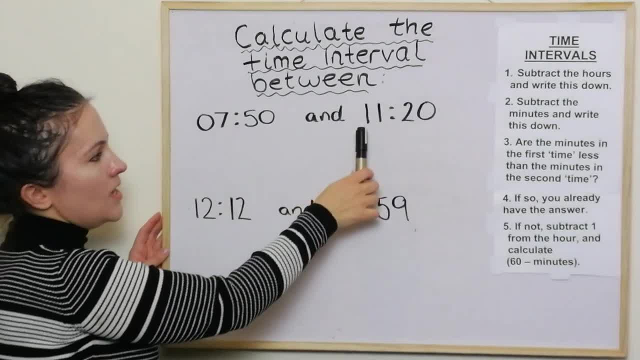 how long it would normally take. But we'll imagine we're leaving Glasgow at this time and we're arriving in Inverness at this time and we're going to work out the journey time. So we'll just go through the steps. 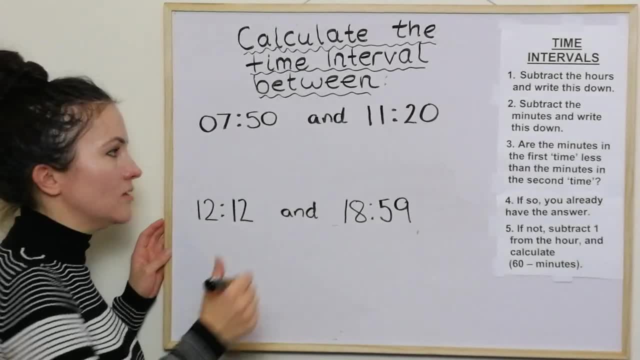 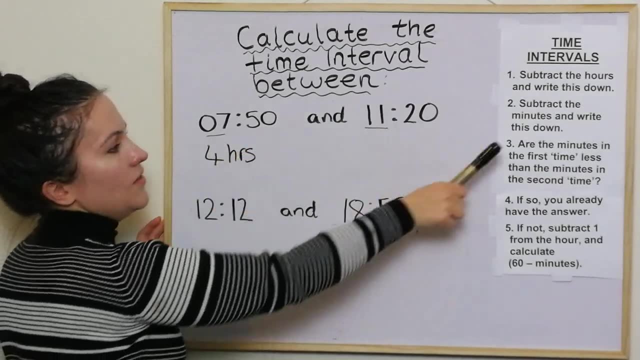 So the first step is to subtract the hours and write this down. So we're just doing the 11 take away seven, That's four hours. And in the next step we subtract the minutes and write it down. So 50 take away 20 is 30.. 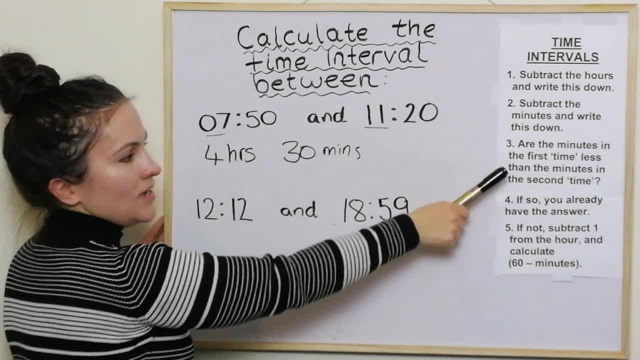 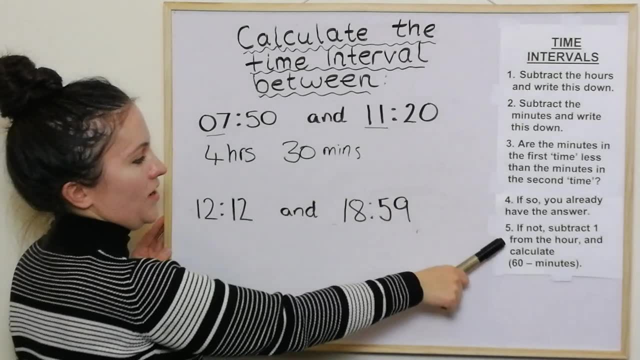 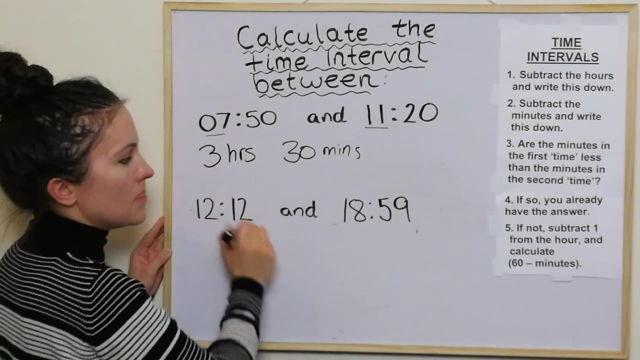 And then it asks: are the minutes in the first time less than the minutes in the second time? Well, the answer is no, So we're going to step five. So if not, subtract one from the hour, So that will become three. 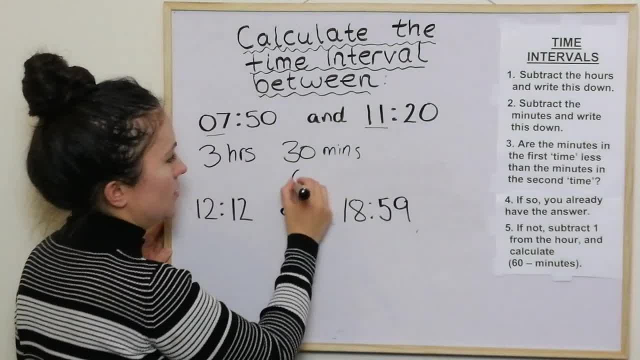 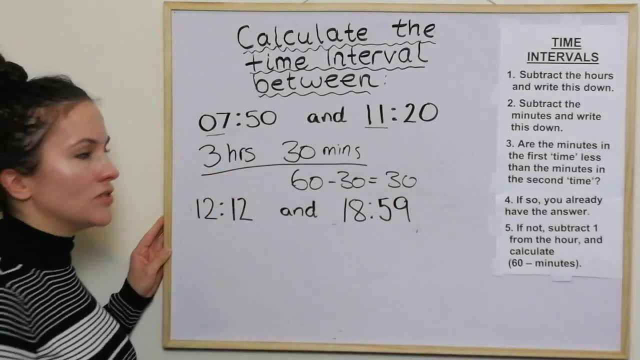 And then calculate 60, take away that number. So 60 take away 30 is in fact just 30. So we already have our answer there. So that would be three hours and 30 minutes, This one here. well, imagine a train this time. 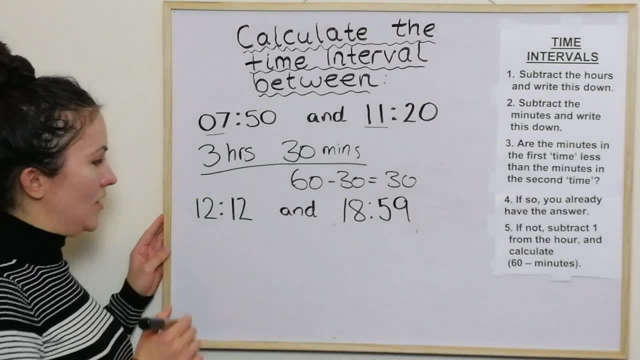 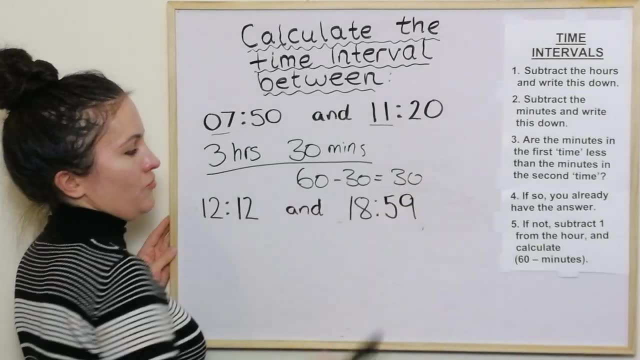 going from Edinburgh to London. And again, it's not based on accurate times. I've just made this up, So we go through the stages, You subtract the hours and write this down. So we've got 18 and we've got 12.. 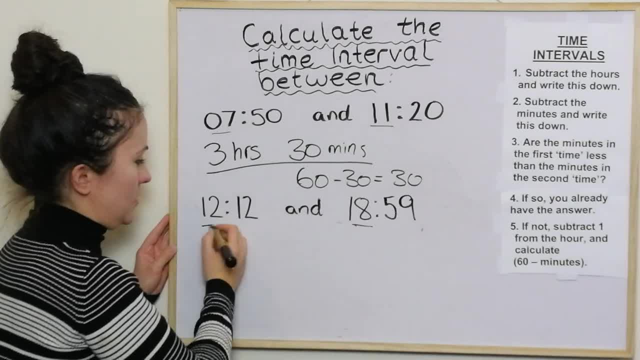 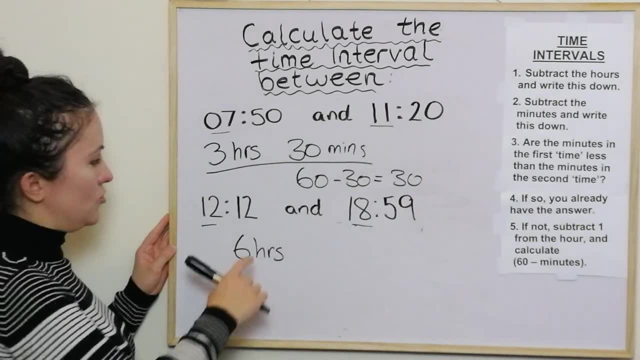 So we subtract them from each other and we get six hours. And that's the first step. Then we subtract the minutes, So we do 59 take away 20.. And then we subtract the minutes, So we do 59 take away 20.. 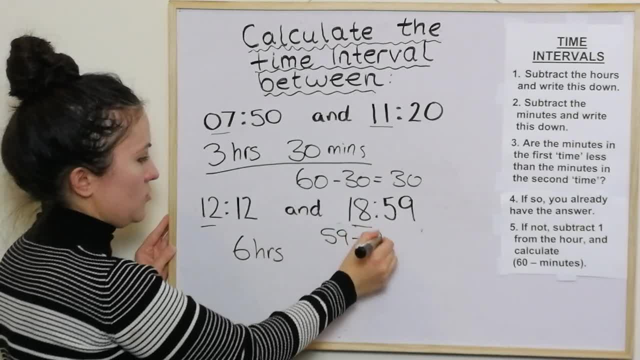 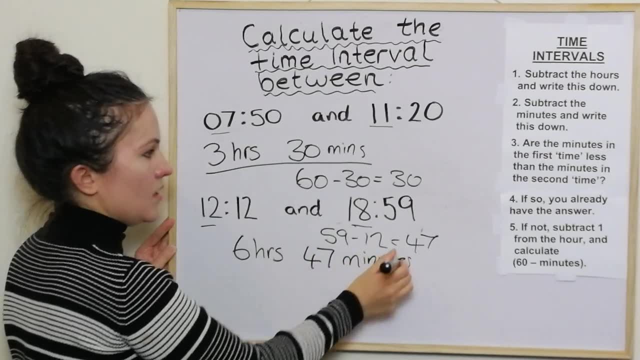 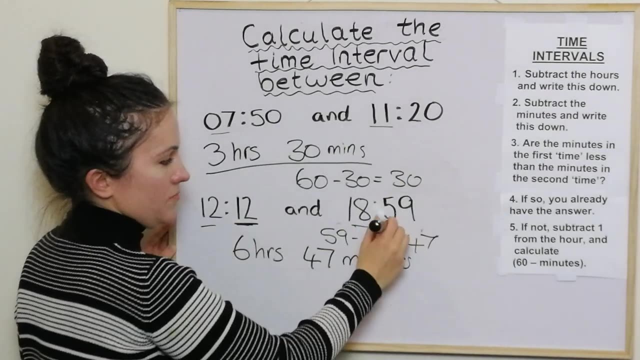 So we subtract the minutes, So we do 59 take away 20.. away 12.. So 59 take away 12 is 47. So I'll just write that down: 47 minutes. And are the minutes in the first time less than the minutes in the second time? Well, yes, because 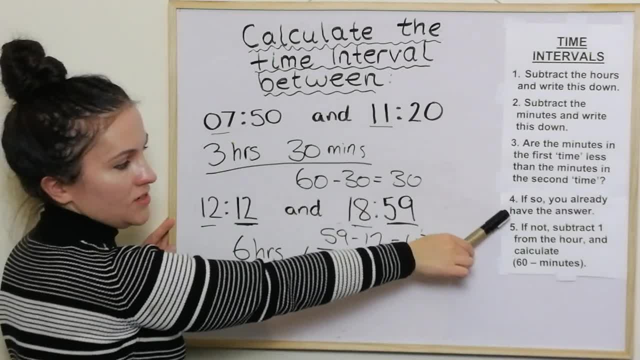 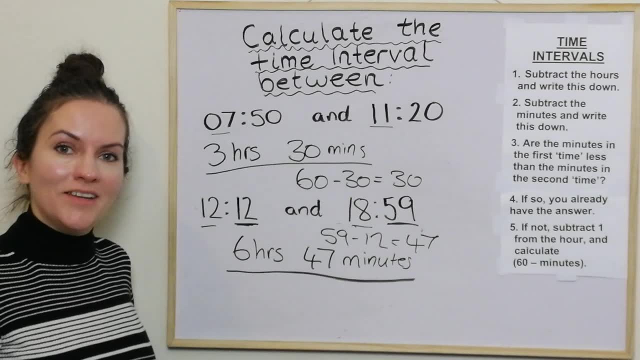 12 is less than 59. So in this case, we already have the answer. So it's 6 hours and 47 minutes. Okay, I'm going to give you a couple to try, Okay. so what I'm going to. 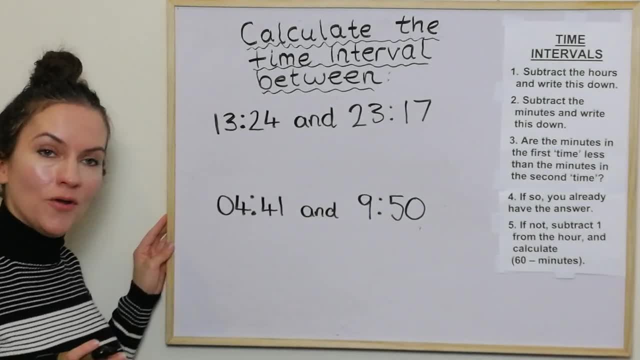 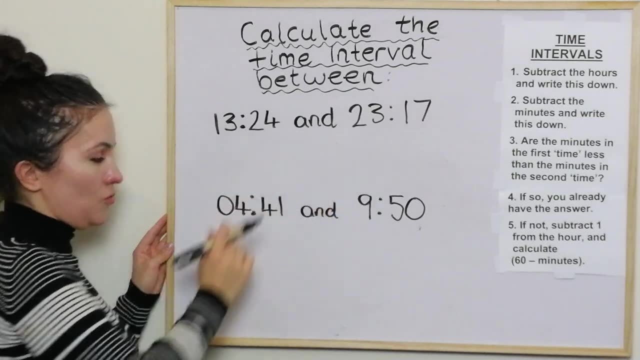 do is- I'm going to let you try these two yourself and see how you get on. So what to do is just pause, get a screenshot, make sure you have the list of steps and we've got this time interval to work out and this time interval to work out. We'll pause and then I'll go. 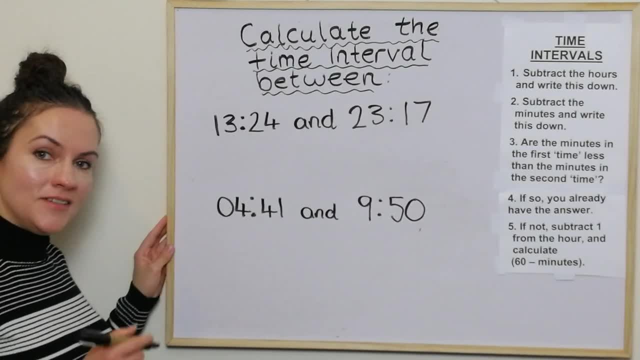 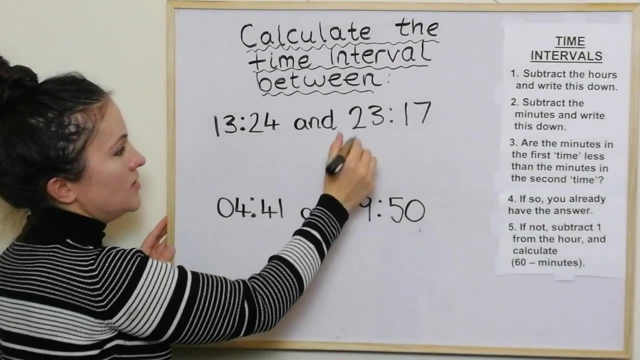 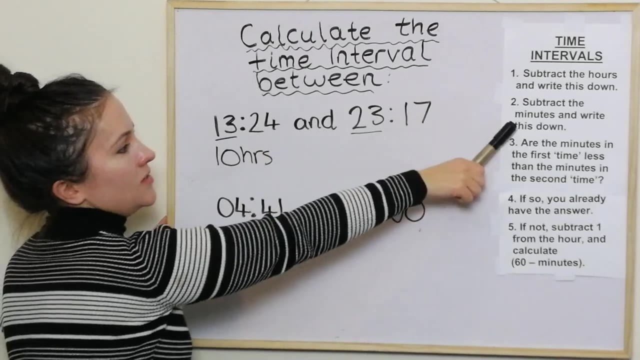 over it. Let's see how you got on. So in this first one here I'm going to give you an example. First thing you do is subtract the hours and write it down. So you do 23, take away 13. So that's 10 hours. And the next step: you subtract the minutes and write. 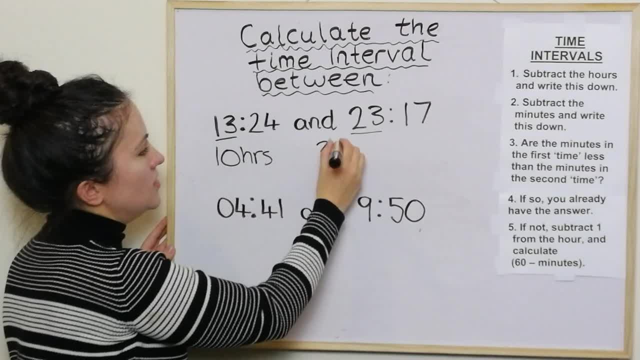 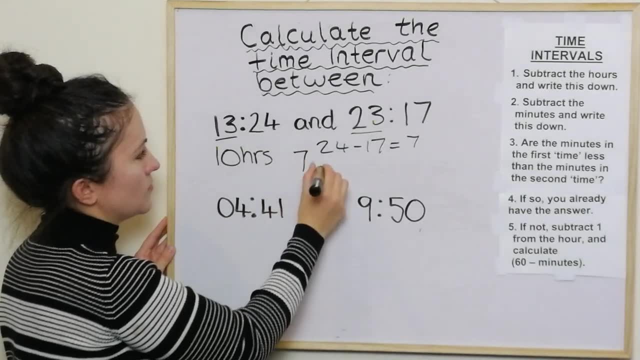 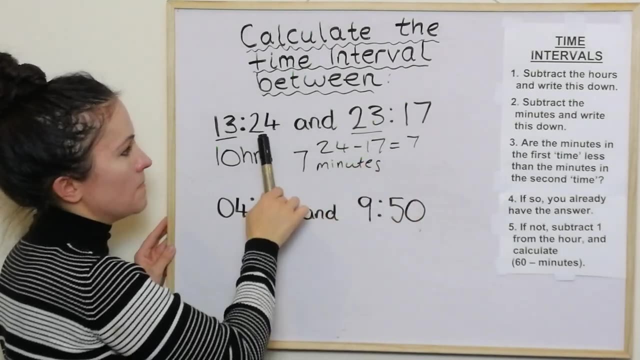 this down. So we've got 24 and we take away 17,, which actually gives me just 7 minutes. So I'll write this down: Are the minutes in the first time less than the minutes in the second time? Well, the answer is no, they're actually more. So what we do is we subtract. 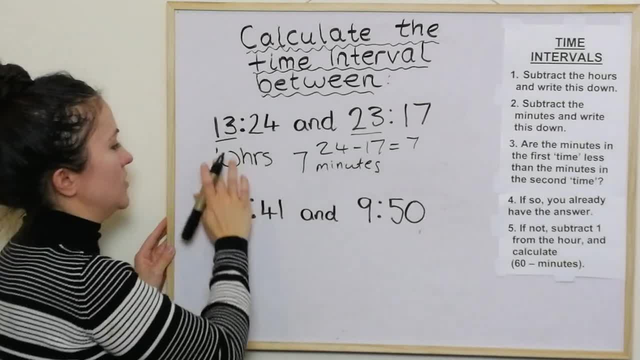 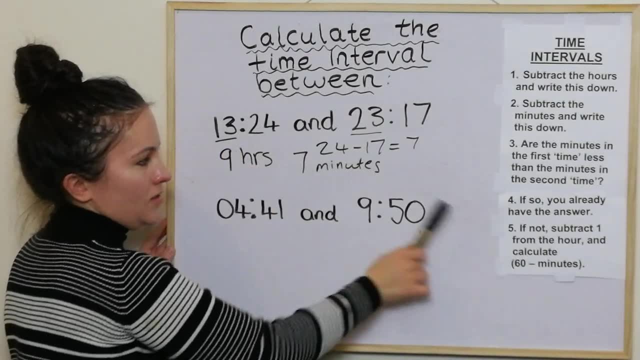 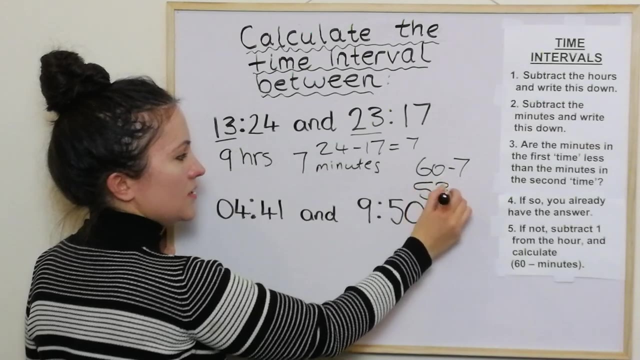 one from the hour, So instead of being 10, it becomes 9.. And then calculate 60, take away 7.. So we do 60 take away 7, which is 53 minutes. So I'll just write that in there. So that's.